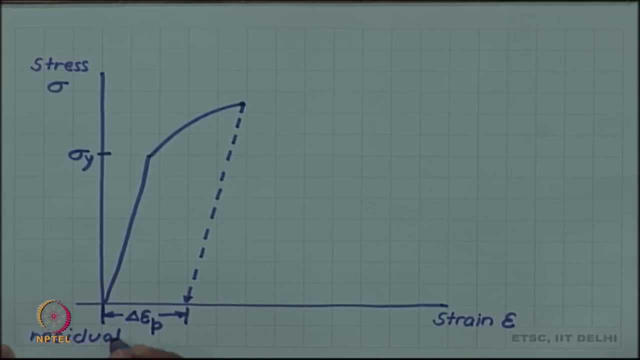 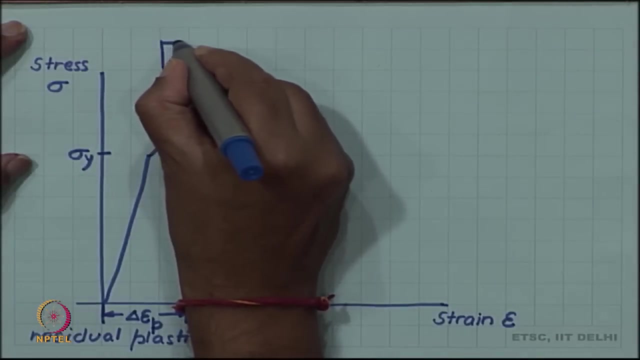 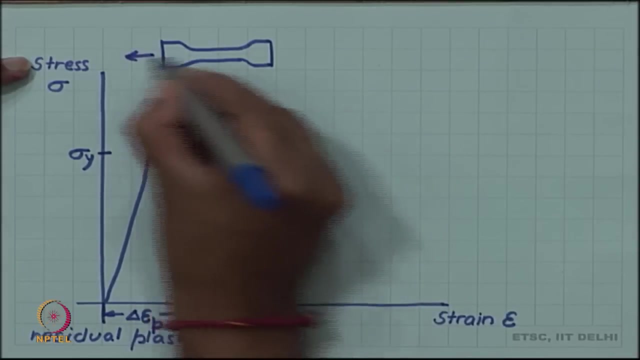 Now let us go to the next slide. So what we have done we started with, remember, our dog bone, kind of specimen for tensile test. So we were pulling this under tension and we were generating this curve. Now, although the sample has plastically deformed, so it is elongated. 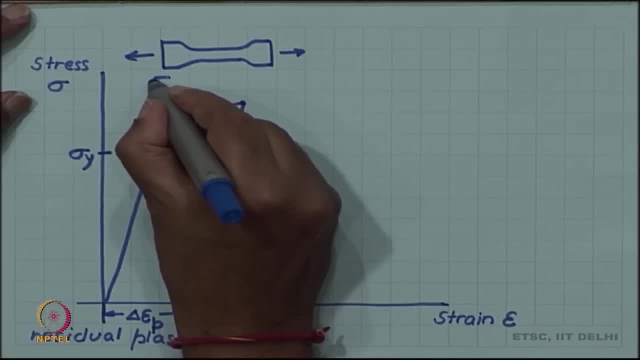 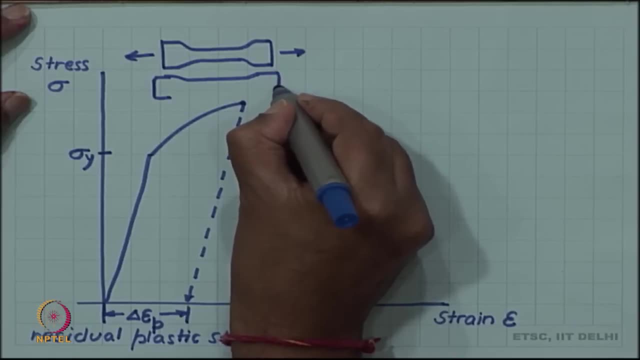 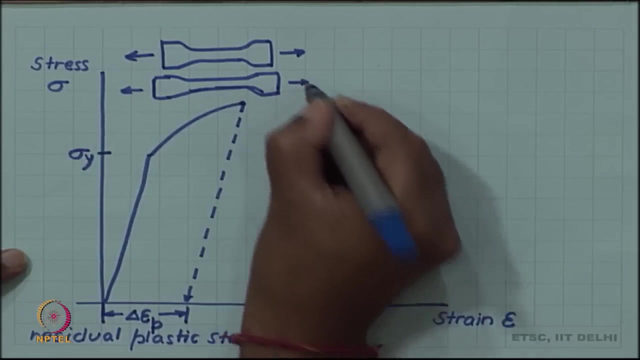 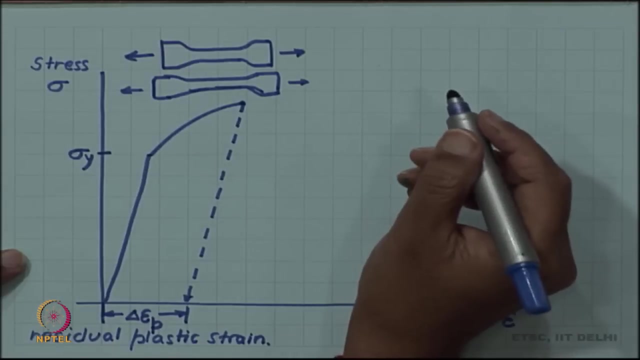 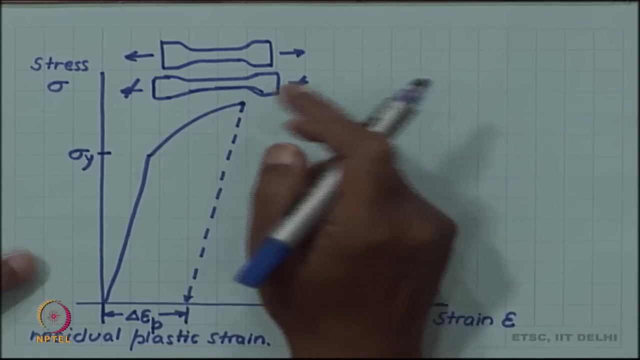 Yes, Okay, Yes. So let me try to draw the deformed sample. so it is slightly longer now and may be diameter is also little bit reduced, but otherwise the sample is still intact. so this is the unloaded specimen. Let me switch off this truss now. so after plastic deformation I have an unloaded specimen. 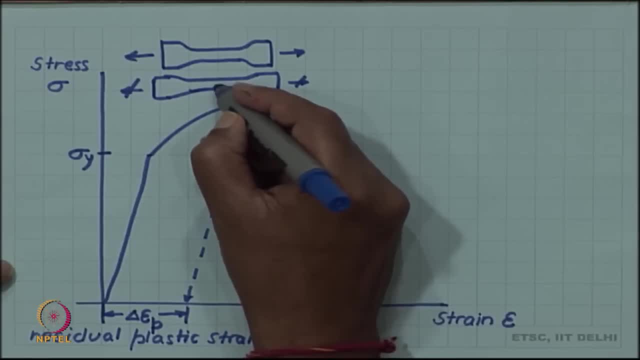 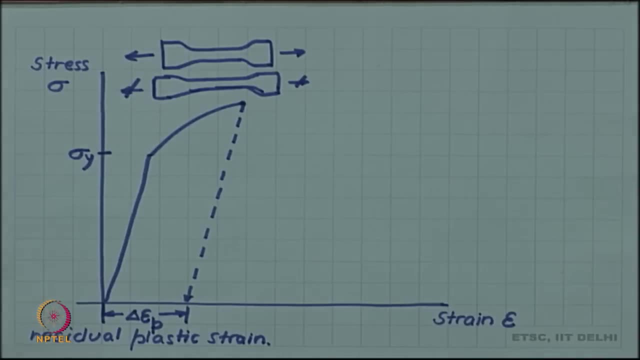 which is little longer and may be a little smaller in diameter than the original specimen. Now suppose, since this specimen is still existing, we have not lost it, it has not broken. suppose we repeat the tensile test on it. On this, what will happen? 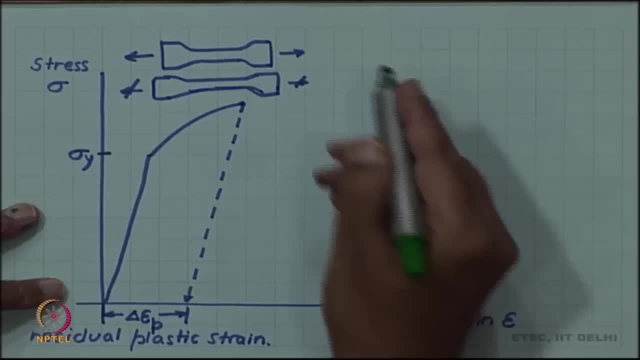 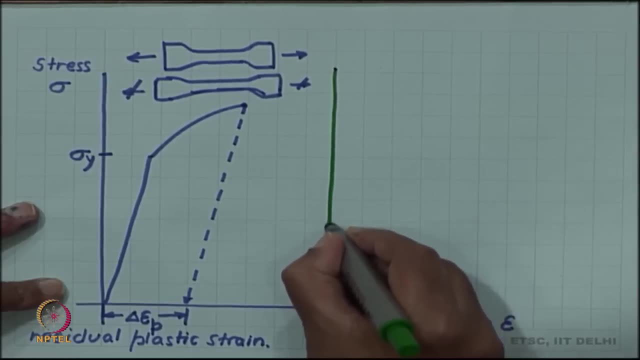 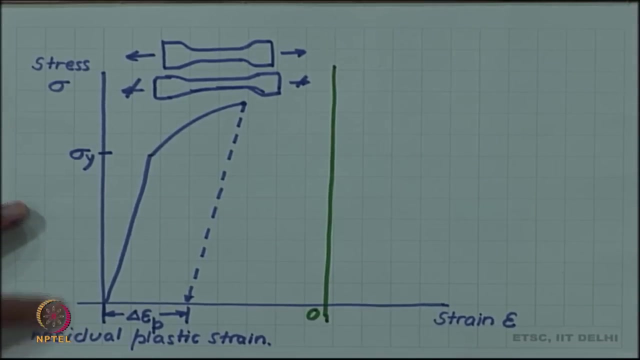 So let me create a new axis for our repeated tensile test. so we are shifting the origin. so now I am taking the zero of the strain here, the new zero of the strain here, and we are loading, we are retesting the loaded sample. 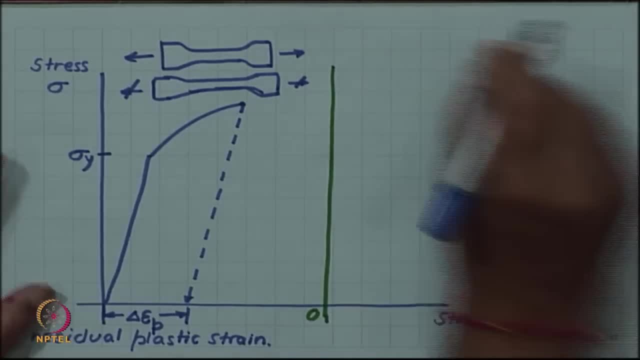 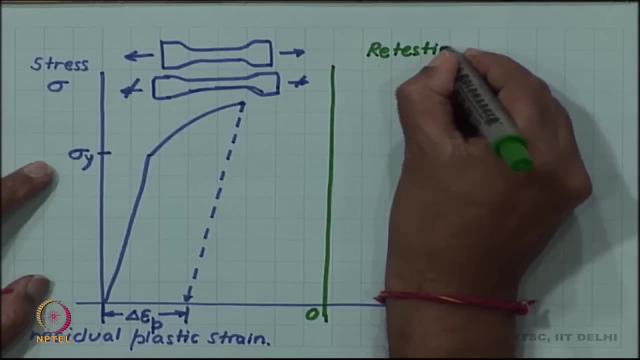 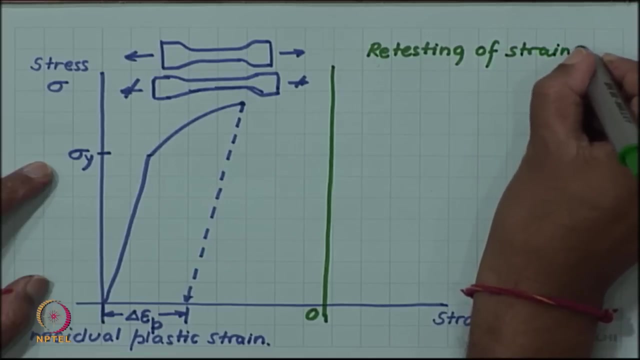 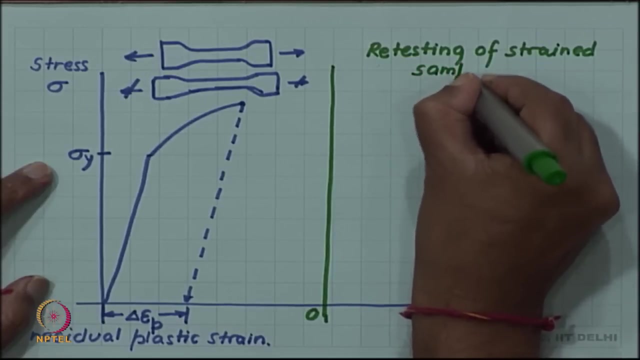 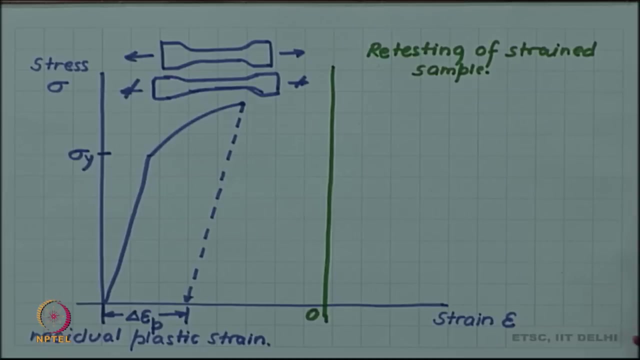 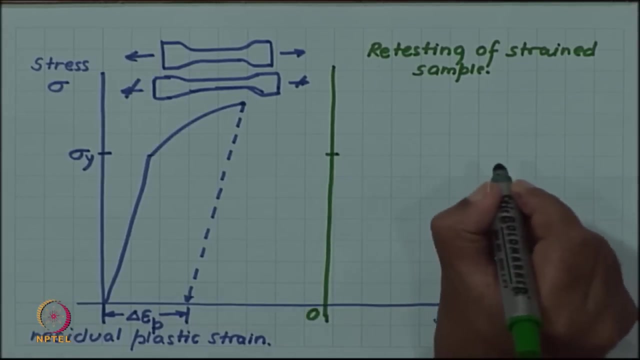 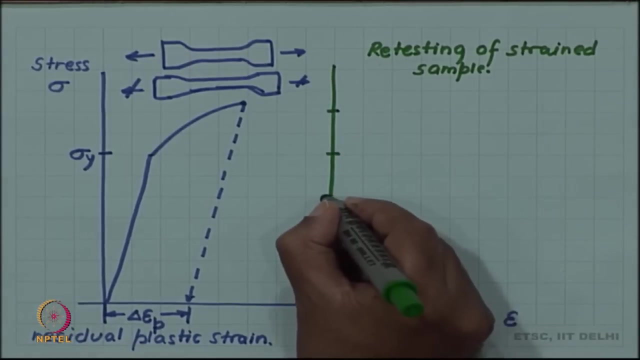 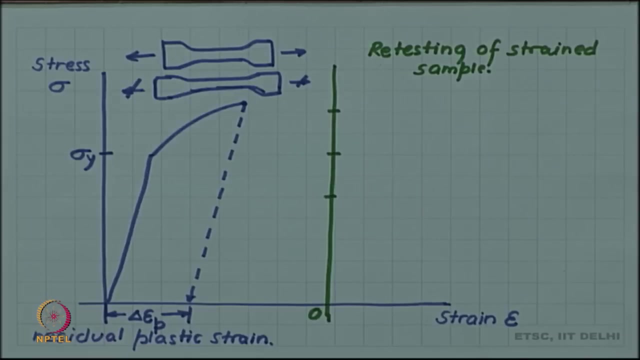 So we are retesting the strained sample, strained or deformed sample. So what we will see, What we will find, That is the question, in particular in terms of the yield stress, will it show the same yield stress, sigma y, or will the yield stress be higher or will it be lower? so that is. 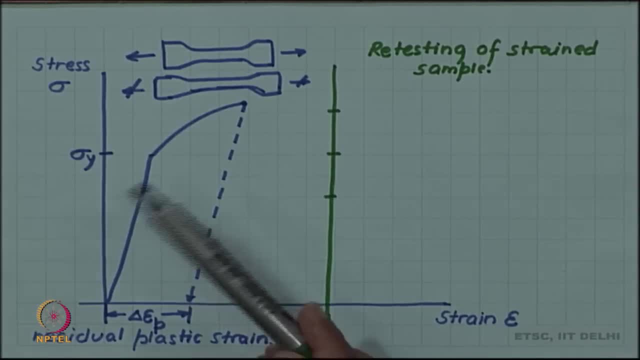 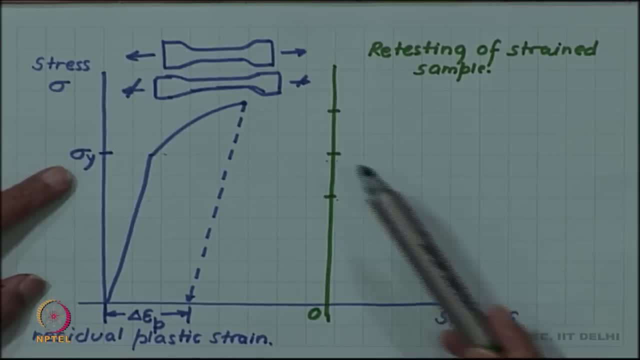 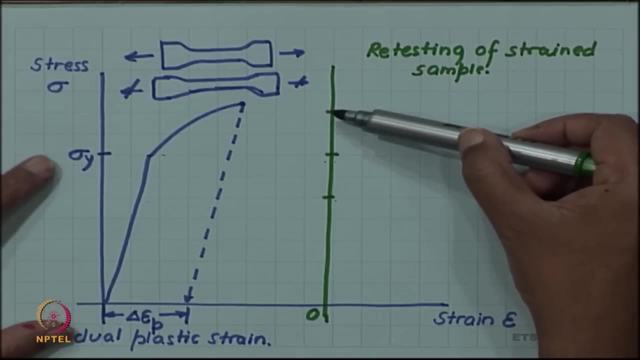 by deformation and remains the same. so yield stress remains the same in the deformed and undeformed specimen? or the final answer that the yield stress is actually larger. you have deformed the material and due to deformation, the material has become stronger. Which of these three options will you choose? 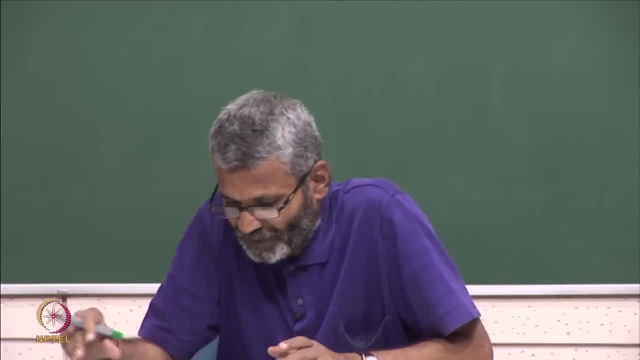 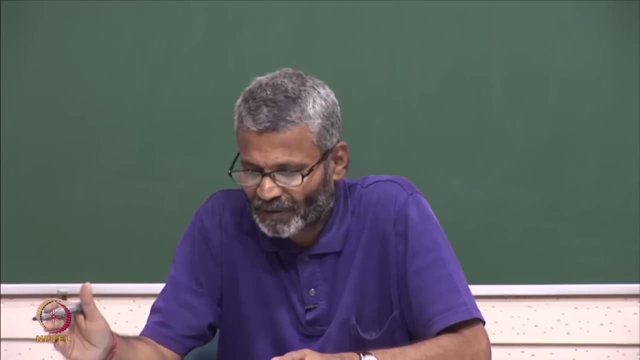 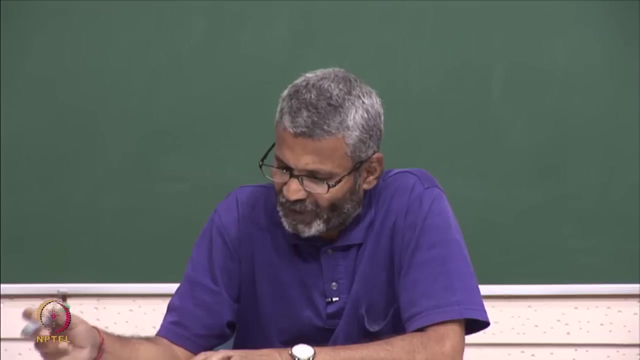 Again. we have seen again and again in this plastic, particularly in this plastic deformation chapter, that such questions cannot be answered philosophically. you have to actually do the experiment and find the answer. so we propose the question to the nature, so we actually do the test again. 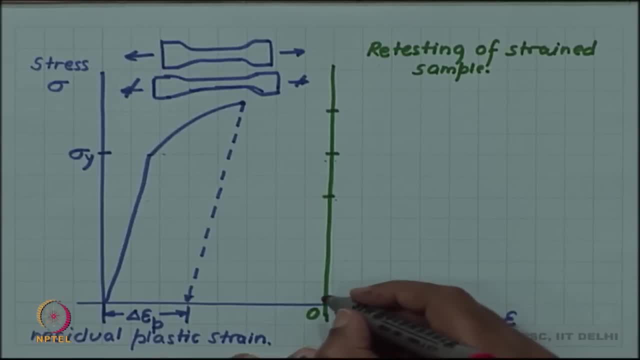 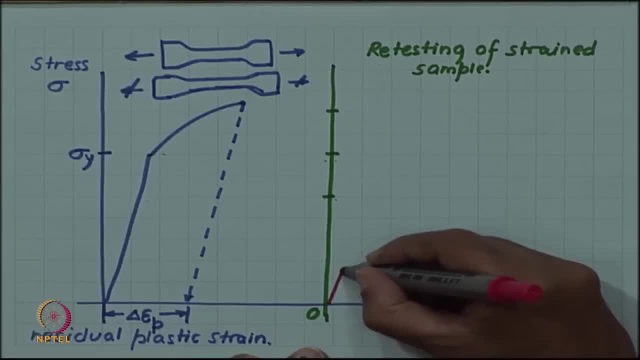 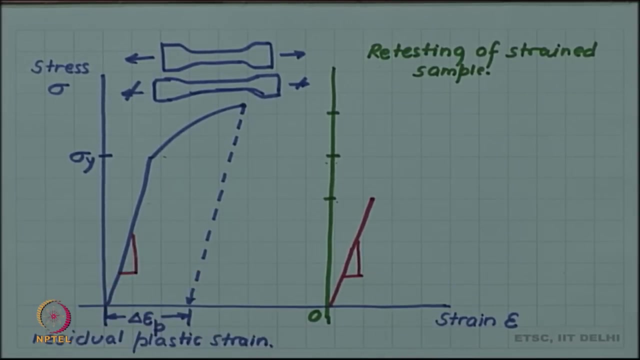 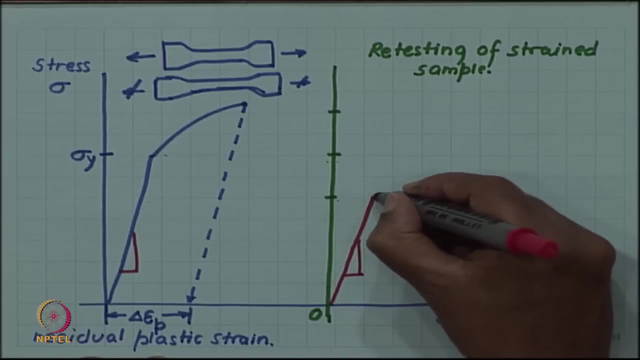 What we find. first thing, we find that the slope of the stress strain curve does not change, So the modulus is exactly the same. So there is no effect of straining or no effect of deformation on the modulus. however, the curve does not change. 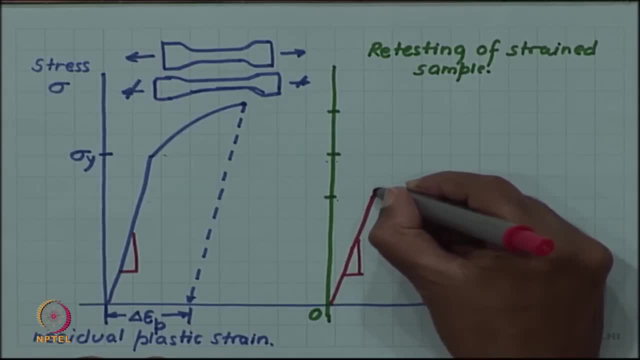 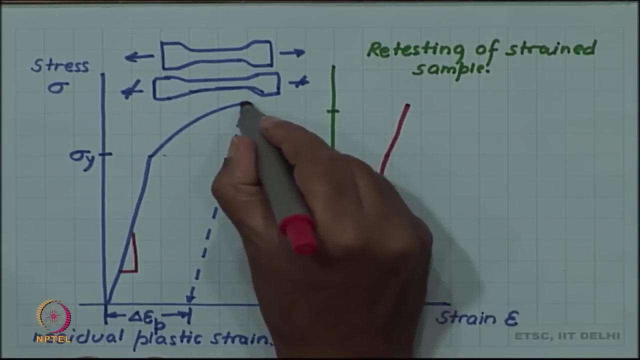 So a deviation from linearity, or it does not undergo plastic deformation at a stress lower than the original yield stress. So it continues up to the original yield stress, but it does not stop there. it continues further beyond, up to the point where you have started unloading. 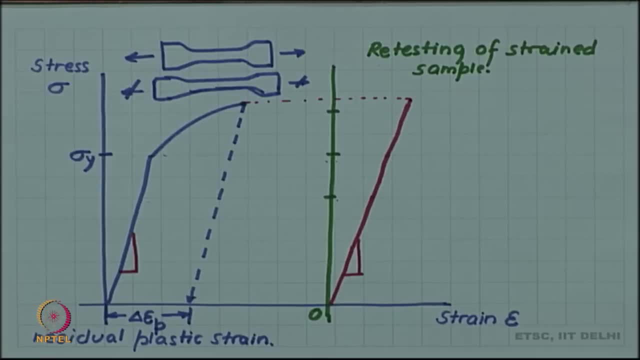 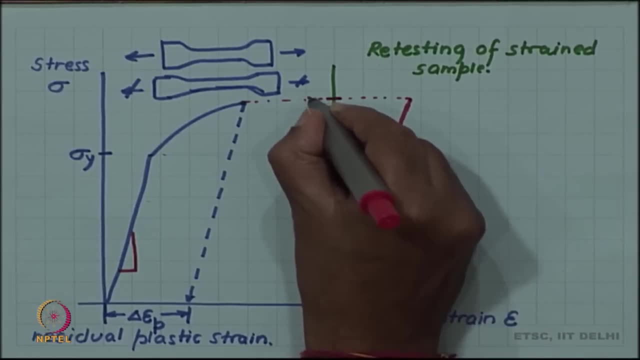 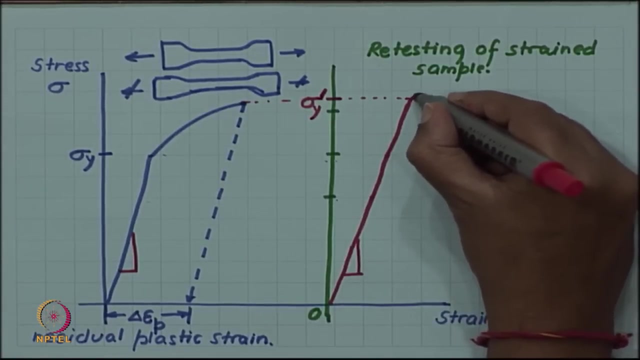 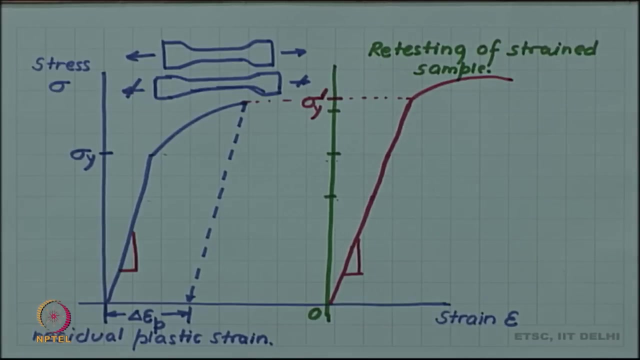 So it sort of remembers its point from which you had unloaded it. so that becomes that point, becomes your new yield stress, and then it continues its plastic deformation. So which means that after deformation, when the test is done on a plastically deformation deformed specimen, the deformed specimen has a higher yield stress than the undeformed. 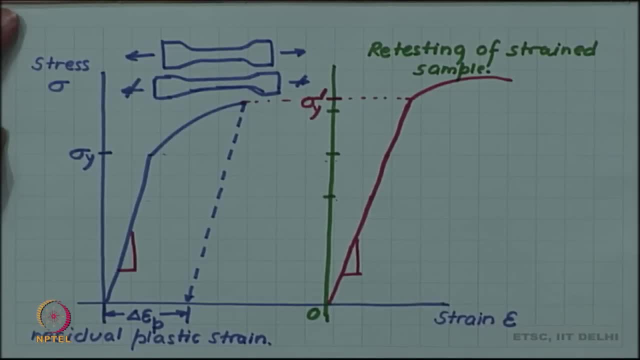 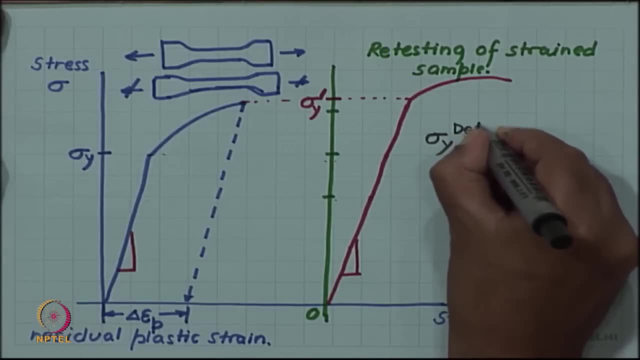 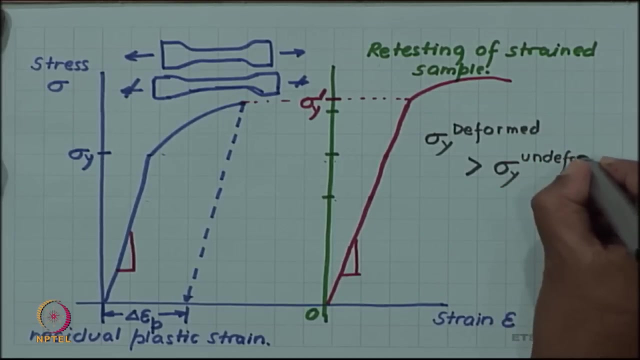 specimen. Let us write this important conclusion: that sigma y deformed is greater than sigma y undeformed. Okay, And this effect? this is the phenomenon which has been termed strain hardening. the question is why it is happening. we will look at that, but at the moment, at the level of definition, 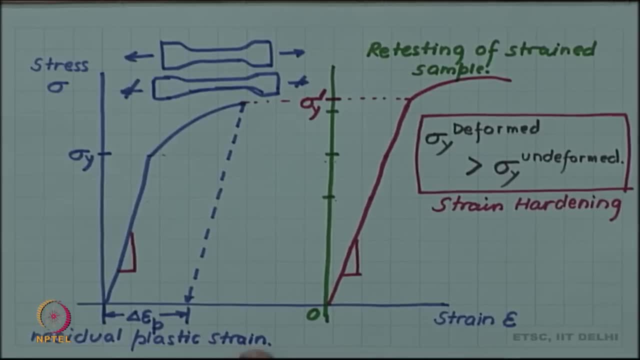 or at the level of observation. what we see is that if a material is plastically deformed and then tested in a uniaxial tensile test, it will show a higher yield stress than an undeformed specimen. So in a way, this plastic strain. what was the difference between the red curve and the 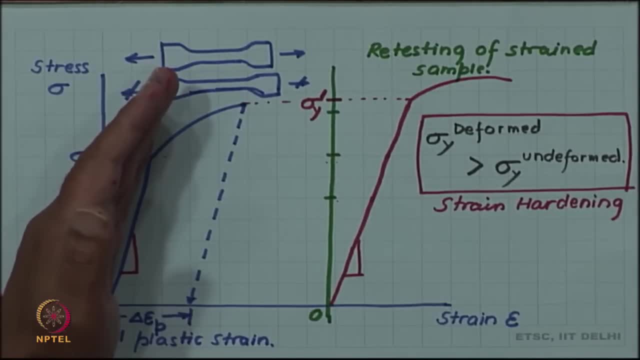 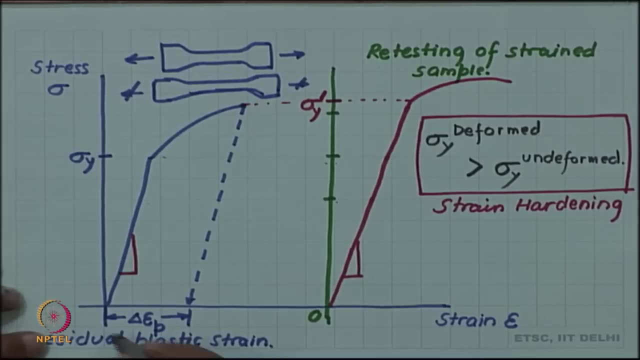 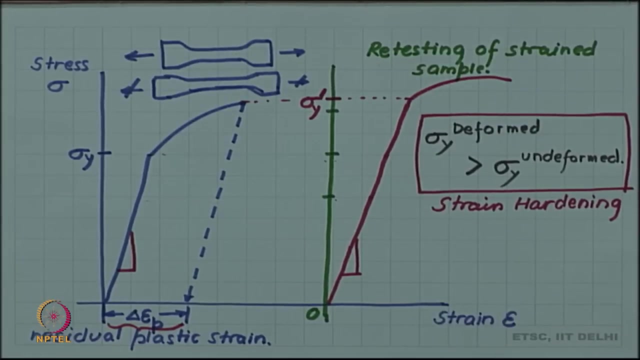 blue curve. The blue curve was originally tested and had no plastic strain, whereas the red curve has an inbuilt. this much amount of plastic strain is already there in this and it is. that is why this is called a strain hardening. In engineering it is also called sometimes work hardening because process of plastic. 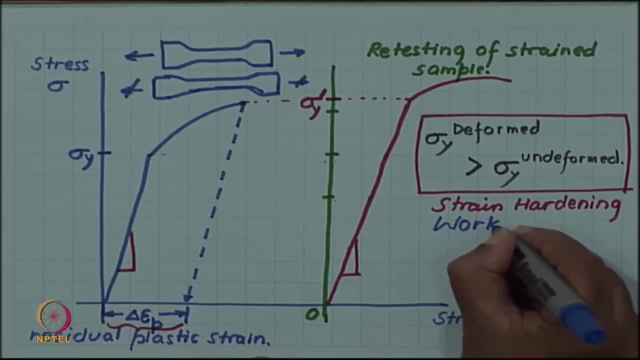 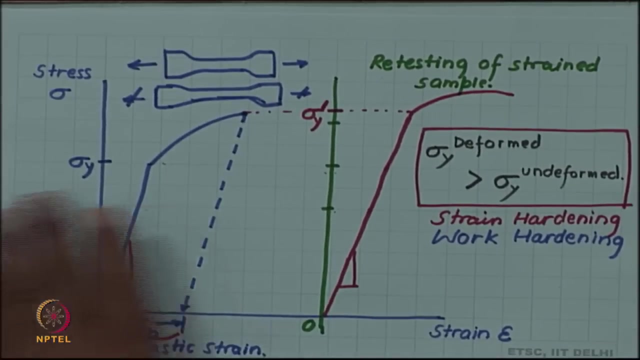 deformation engineers call cold working or working, So it is also called work hardening. Okay, So strain hardening and work hardening are synonyms. Now let us think of it, since plastic deformation is involved, dislocations are involved. so 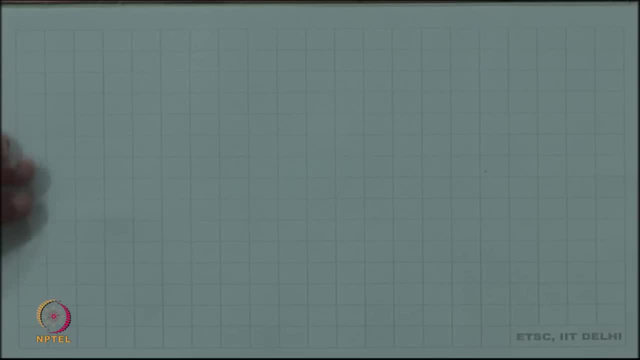 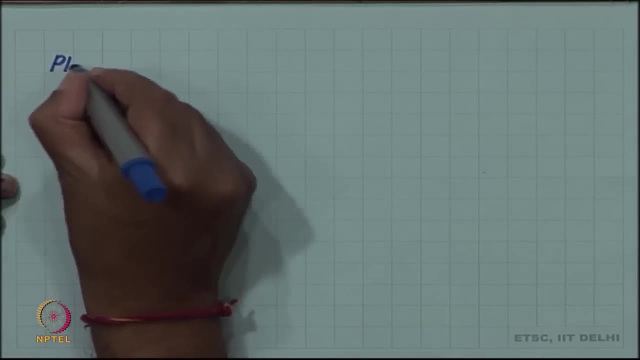 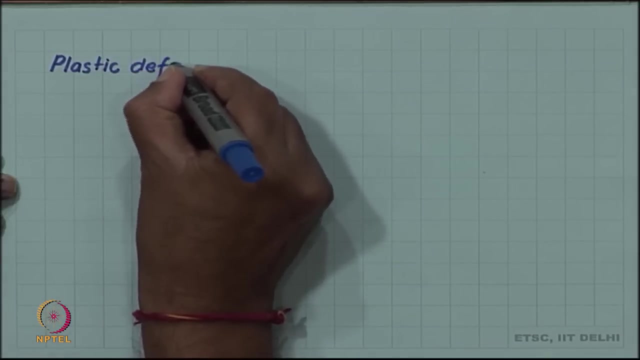 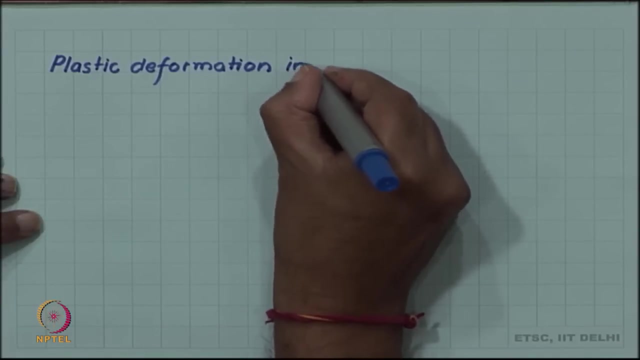 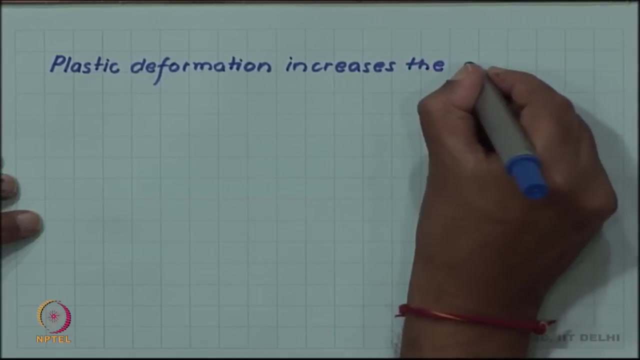 let us look, think of it in terms of dislocations. So we have already seen that plastic deformation. It increases the amount of dislocation in a material, increases the dislocation density And the dislocation density of the material increases the level of the material is increased. 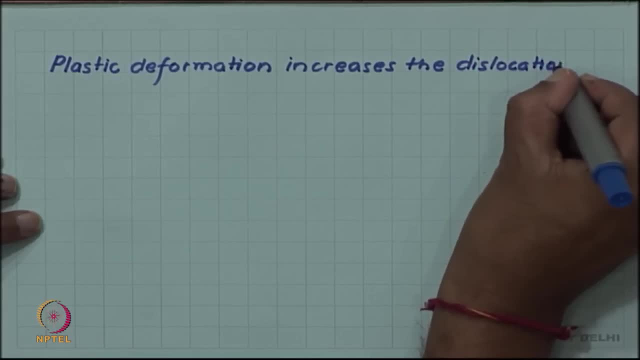 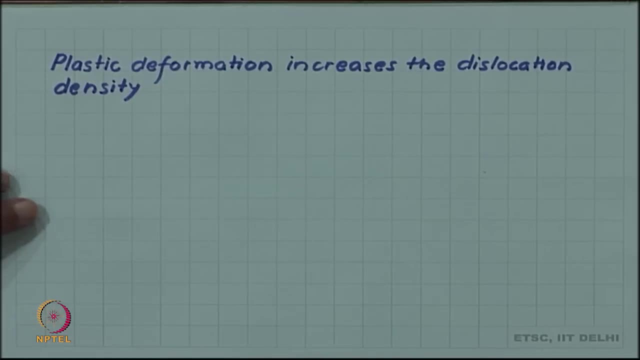 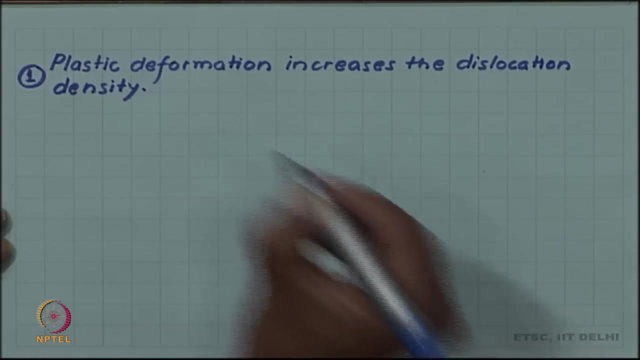 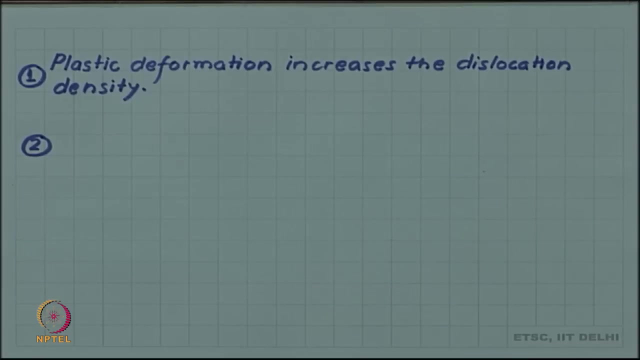 that is the dislocation density, So the material, So the material, The material. But we have also seen, and that is how the dislocation was proposed in the literature of science, as a mechanism or as a device by which you can deform the material at much. 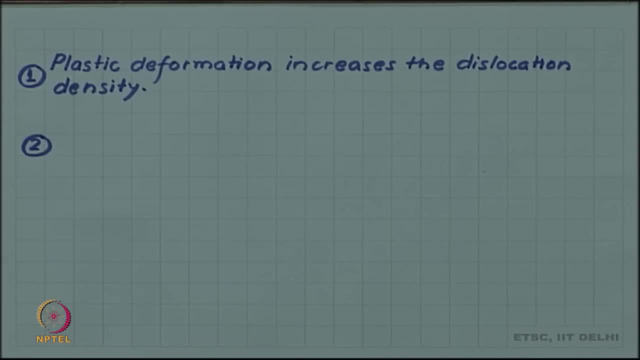 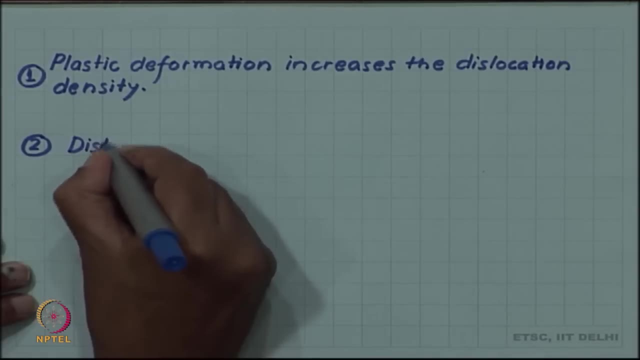 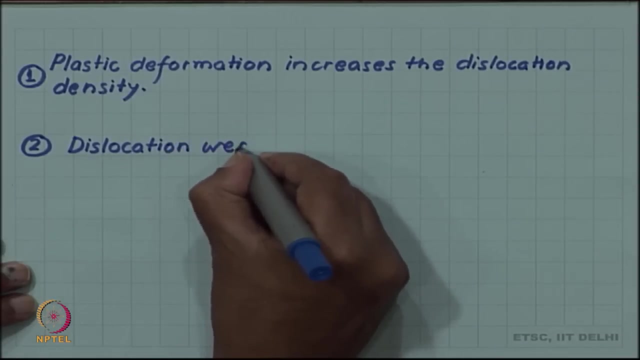 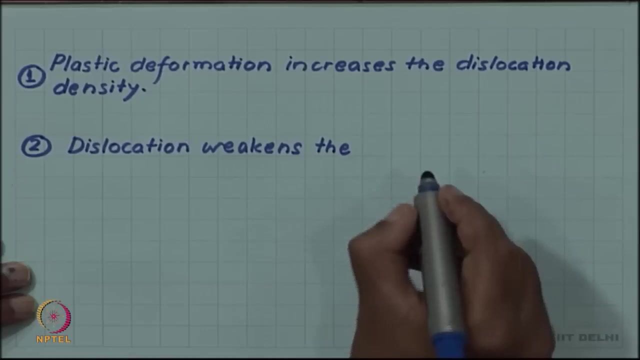 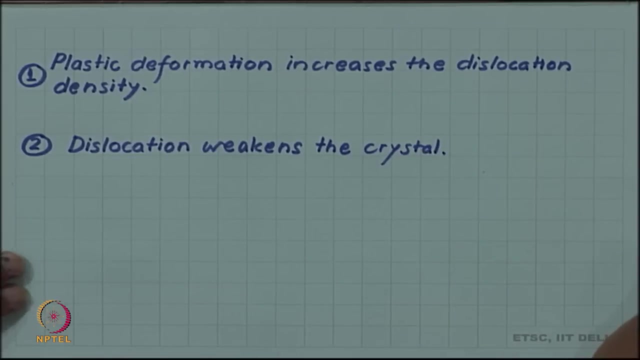 lower stress than the ideal or perfect crystal. So we have also seen that dislocation weakens the crystal. So we have also seen that dislocation weakens the crystal. So if you put 1 and 2 together, the normal conclusion will be: dislocation weakens the. 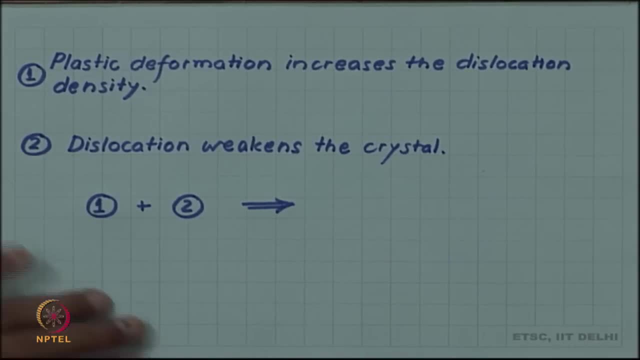 crystal plastic deformation is generating more dislocation density, so deformed crystal should be weaker. So if you put 1 and 2 together, the normal conclusion will be: dislocation weakens the crystal. but we have seen that this is not true experimentally. not true this conclusion. 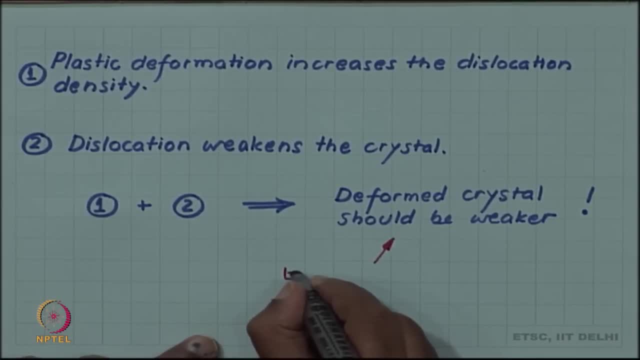 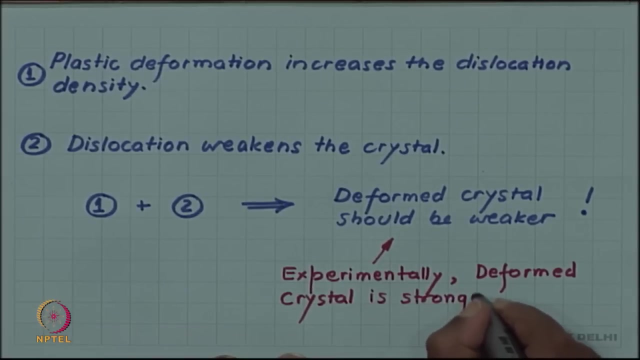 is incorrect. Thank you, Thank you. experimentally deformed crystal is stronger. that is what we call strain hardening. So then, how do we resolve this conundrum, this problem that dislocation is weakening the crystal? we are generating more dislocation during plastic deformation- still crystal.